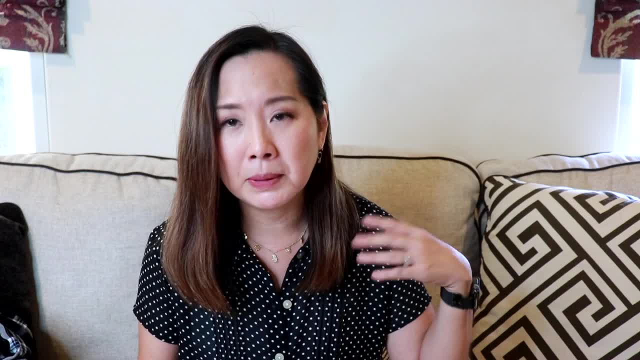 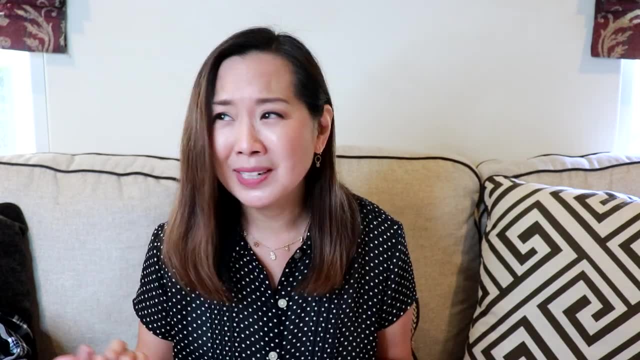 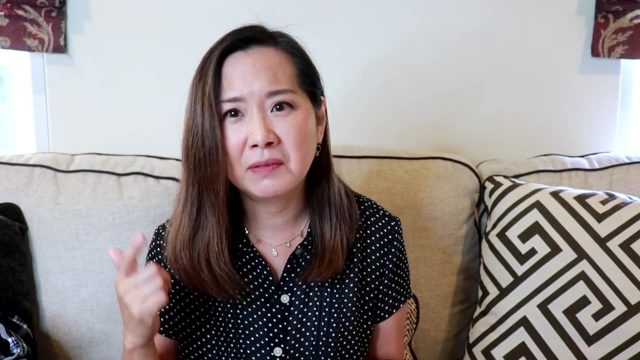 out to one point: six, one, eight, oh, three, three, nine, eight, blah, blah, blah, blah, and goes on and on. so apparently this Phi or Phi- I'm not even sure how it's pronounced, because some I googled it and in some cases call it Phi and some Phi. but let's just call it Phi, but that's how most people. 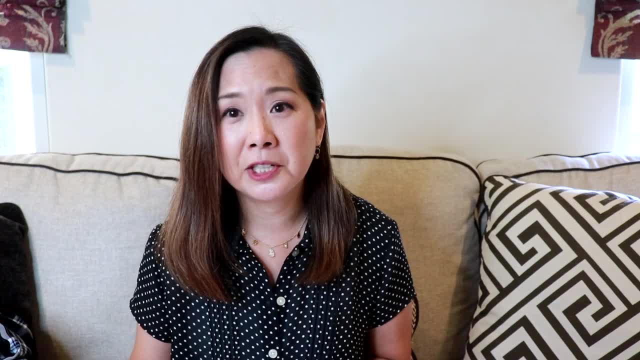 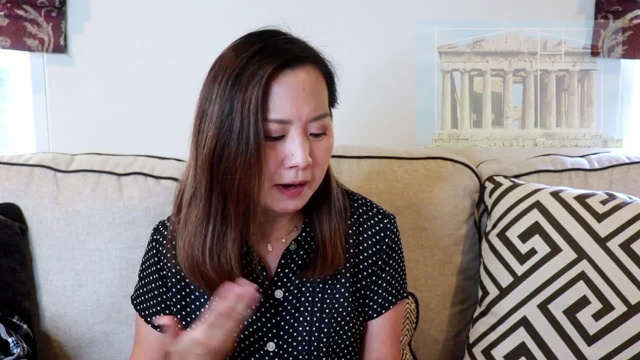 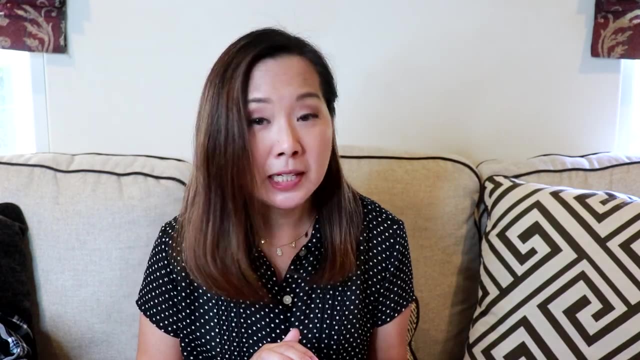 pronounce it? I think okay, but this ratio has actually been used by the Greeks and you can see it in their artwork, also in their architecture, for example, the Parthian, and also even Leonardo da Vinci. he referred to it as the divine proportion and he used it in a lot of his paintings, like for: 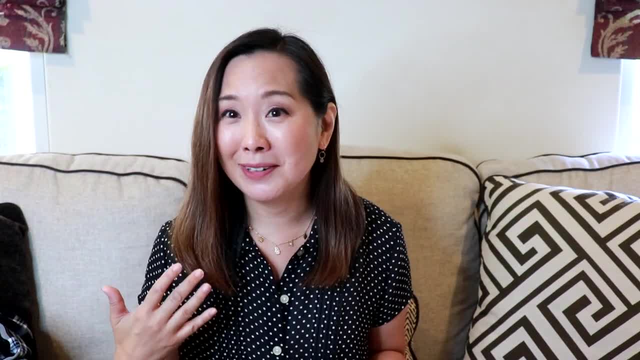 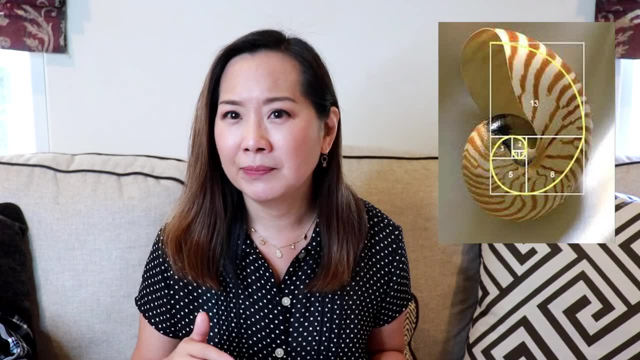 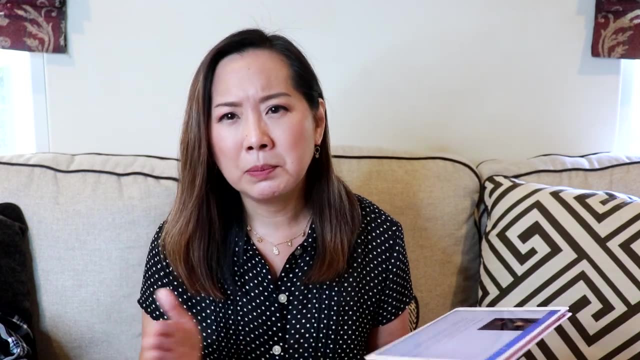 example, the Mona Lisa also, which is also very interesting and beyond the scope of this video. this golden ratio can be found in nature as well, and it's even found in our own DNA, so it's very special, and this proportion is actually something I guess we consider beautiful, and it's just something that we're 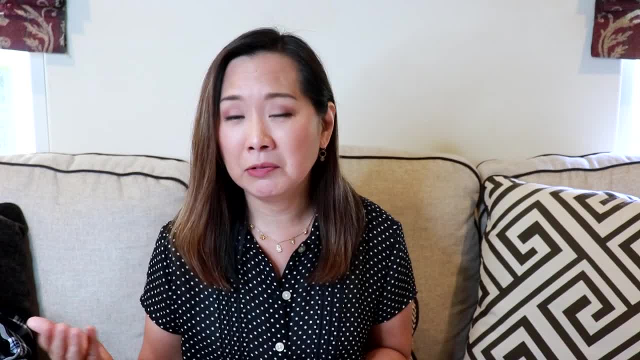 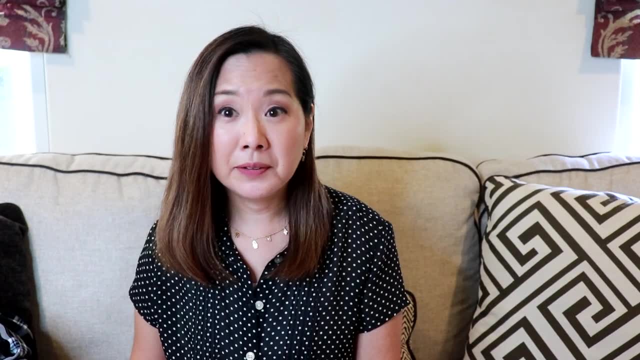 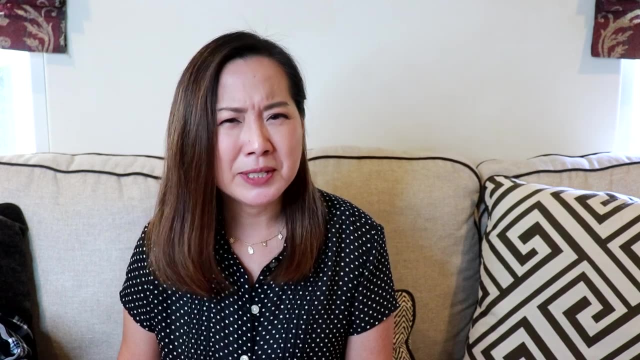 drawn to for some reason. so, even unconsciously, we might be using this golden ratio when we get dressed or whatever, without even knowing it. okay, so now that we have a general idea of what the golden ratio is, you're probably wondering how can it help you dress better? so, basically, what you do is you apply. 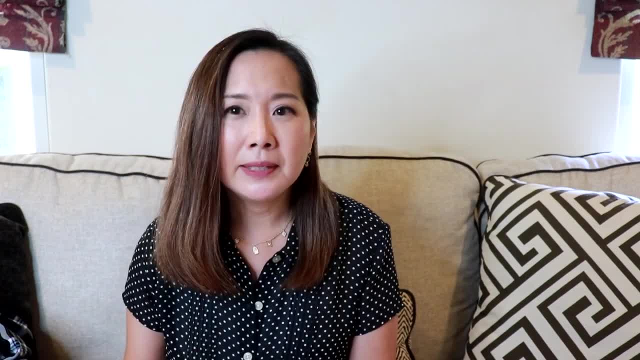 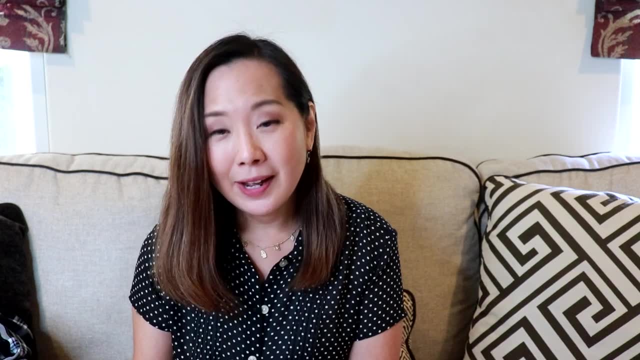 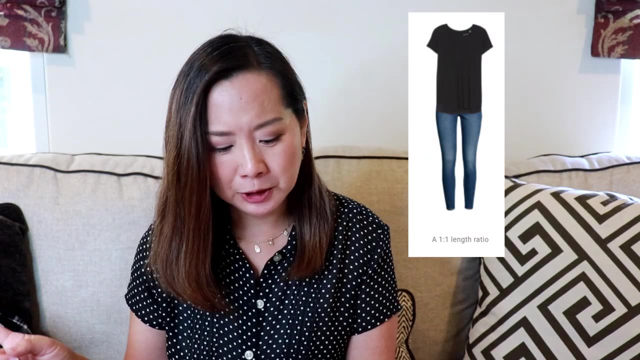 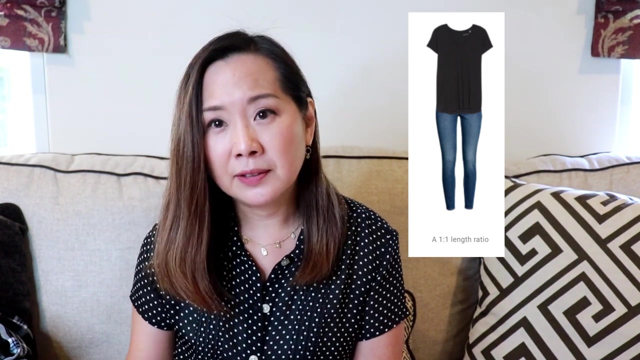 that golden ratio to your outfits. but it's actually easier to understand if you look at some real examples. so I found a couple examples on the internet, and the first is demonstrated with a pair of jeans and a t-shirt. look at the first picture. you'll see that the t-shirt cuts off the body at about the halfway point, so that it's a one to one ratio, and 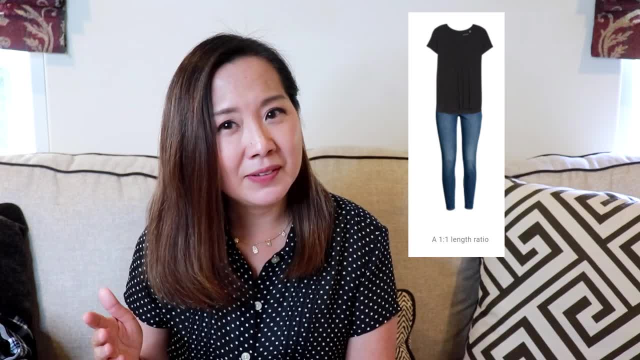 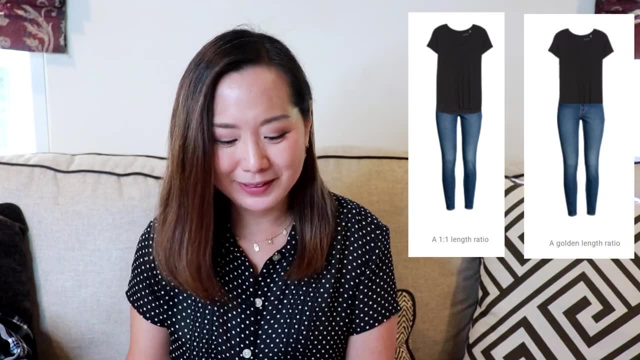 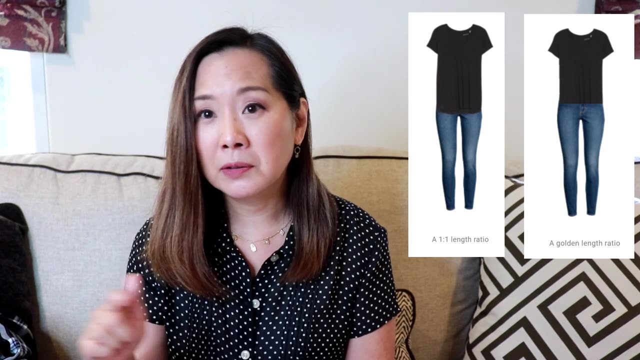 although that's very symmetrical, the eye doesn't perceive that is as beautiful as if you were utilizing the golden ratio. so to make this outfit more attractive, you'll see the set in the second picture. the t-shirt is shortened, which elongates the bottom part, so it's no. 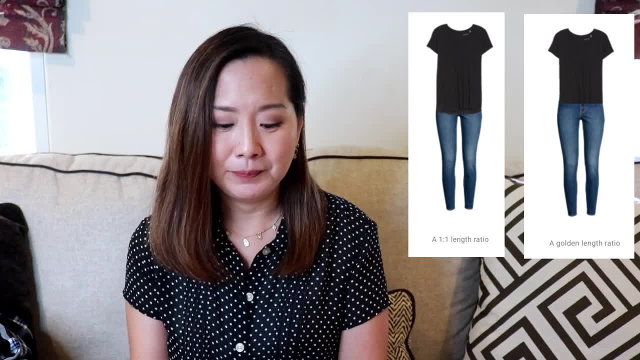 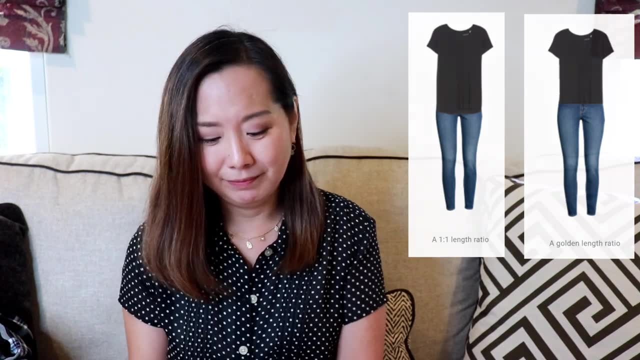 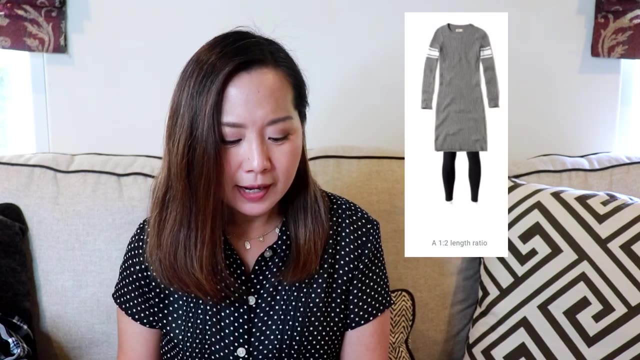 longer 1, two, one ratio, but a one to 1.6 ratio. So yeah, so the second outfit is considered more in line with the golden ratio and therefore more attractive. Okay, let's look at one more example. Okay, so this one is a dress. 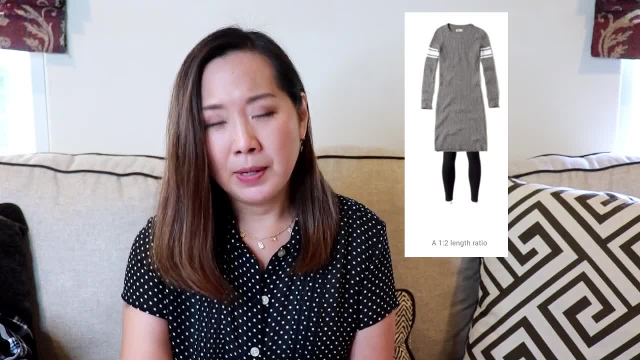 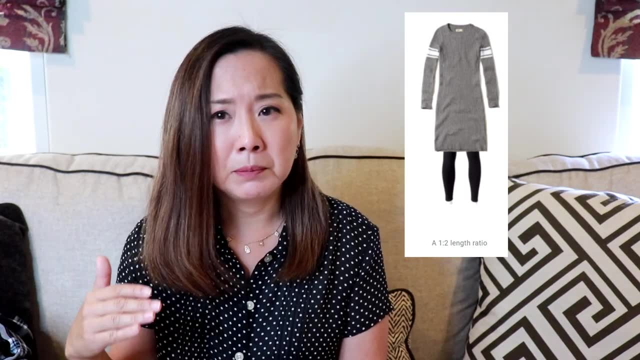 and you'll see that the dress is pretty long and on the bottom there's some tights, So that represents a one to two ratio. So the dress is roughly twice as long as your tights. And to make that outfit look more attractive, 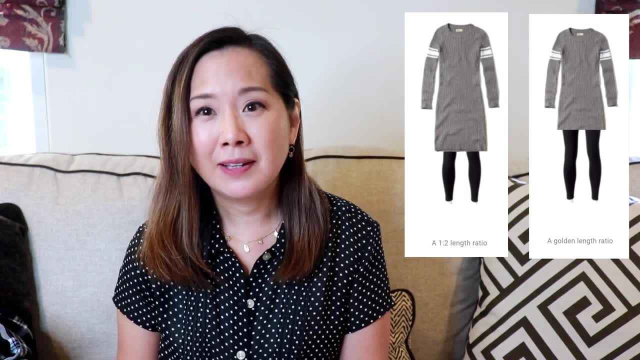 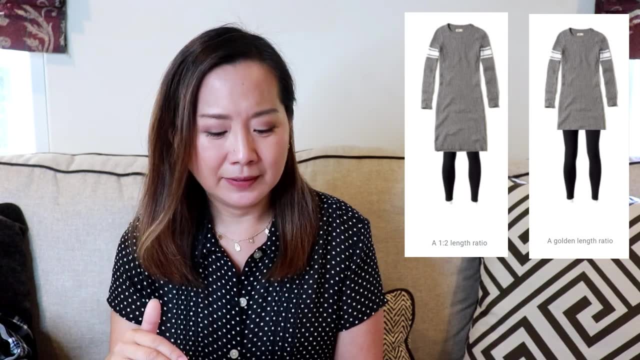 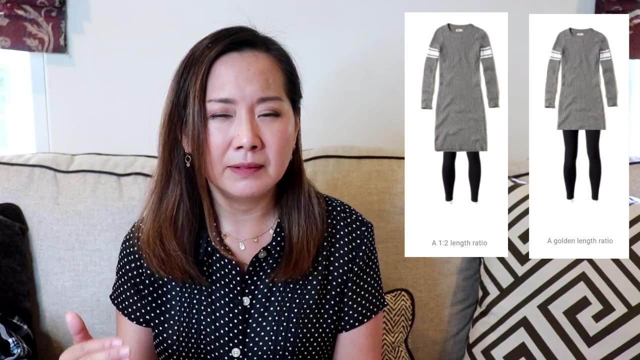 you'll see the second picture, which reflects the use of the golden ratio. So in this case the dress is 1.6 and the tights is one. So that's the ratio: 1.6 to one. So you'll see that it instantly looks better. 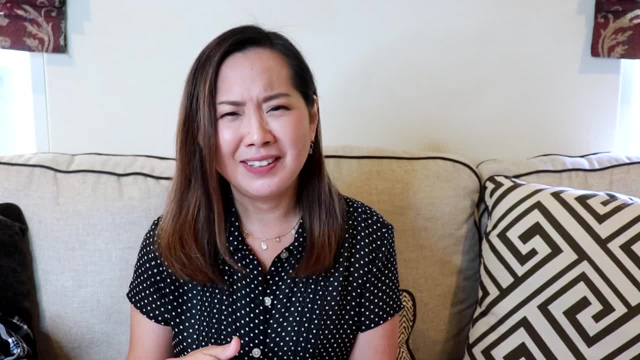 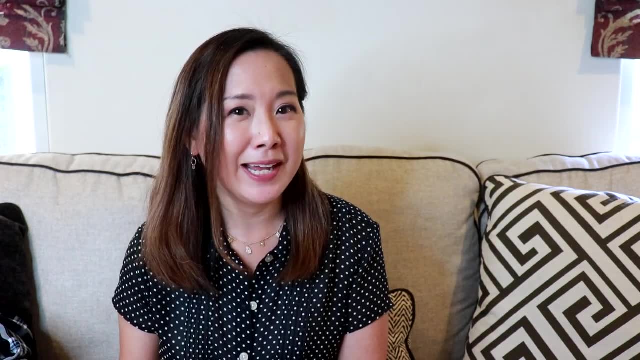 Okay, And there's also a nifty trick that I learned- Did I just say nifty? Oh my gosh. That I learned on the internet, And it's how to calculate your most flattering hemline using the golden ratio. So I thought this was actually really good information. 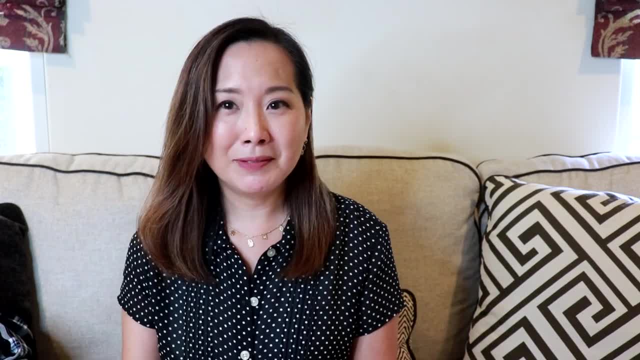 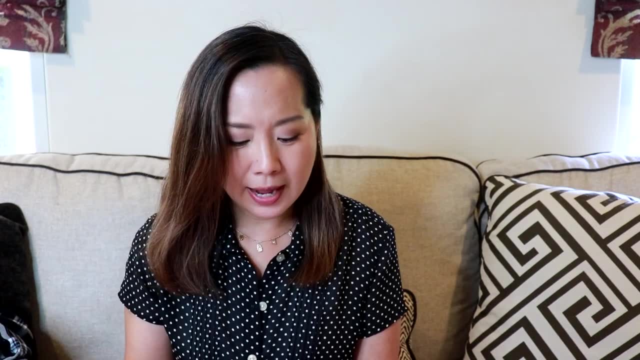 So the way you do it, you actually have to measure your length of your body, and that's from your shoulders to your feet, And I had to get my husband to help me measure. And for me- and I'm 5'1" it came out to 51 inches. 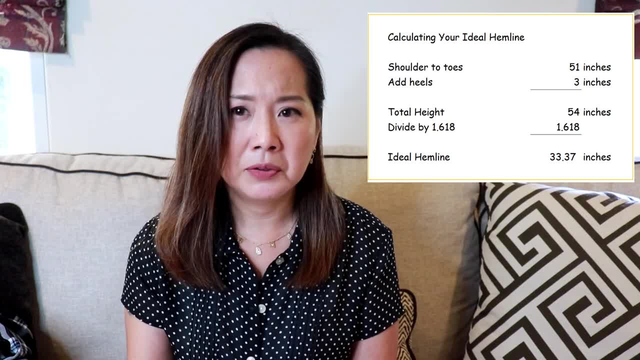 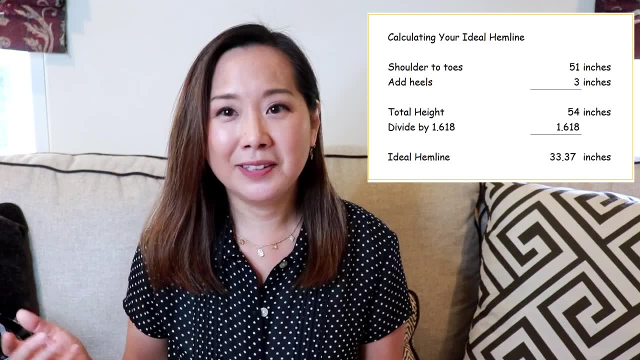 And if you plan to wear heels, you have to add that in too. So usually I wear like three inch heels or wedges, So that my total is 54 inches, And then you take that total and you divide by the golden ratio, which is 1.618.. 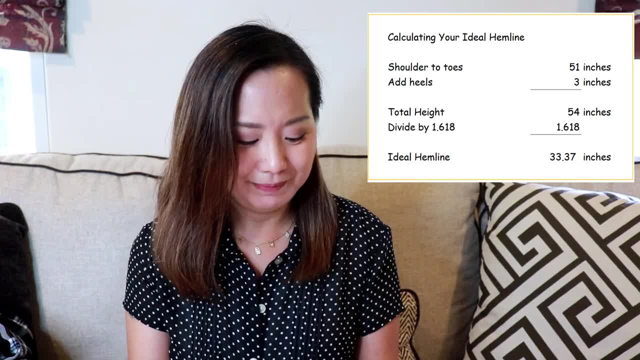 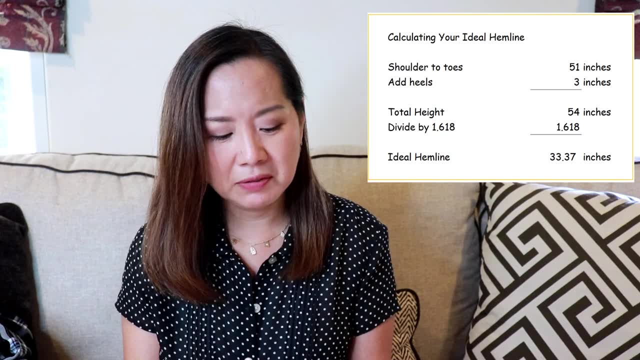 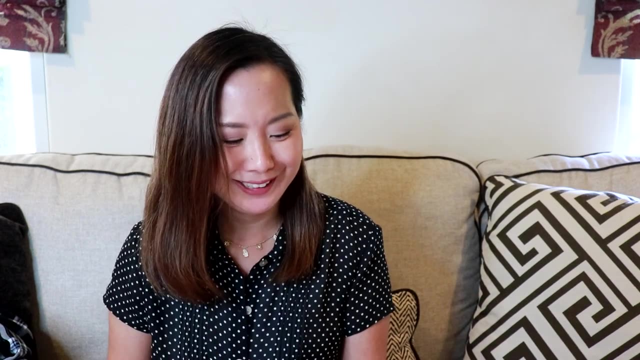 And that result is your ideal hemline. Okay. So for me that ideal hemline came out to 33.37., And that's with heels. If I were to wear flats, it was 31.52.. So I thought that actually seemed a little short. 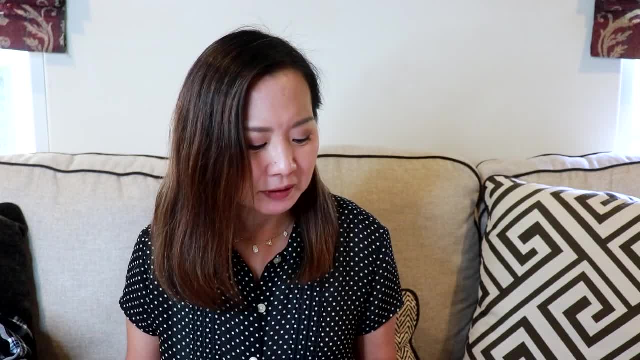 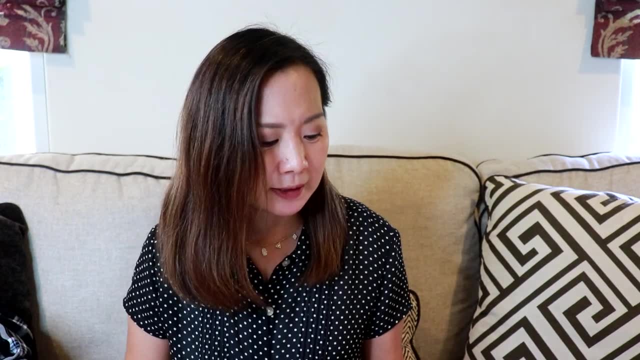 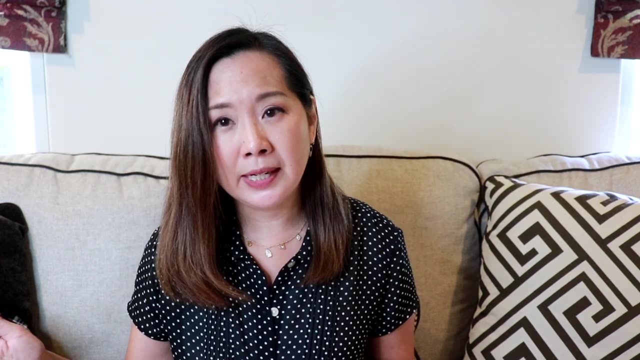 So I would say, yeah, that might be the most flattering length for me, but probably practically I'll have to increase that by a couple inches. And I've also seen online that people generally apply the golden ratio by, instead of a one, to 1.618,. 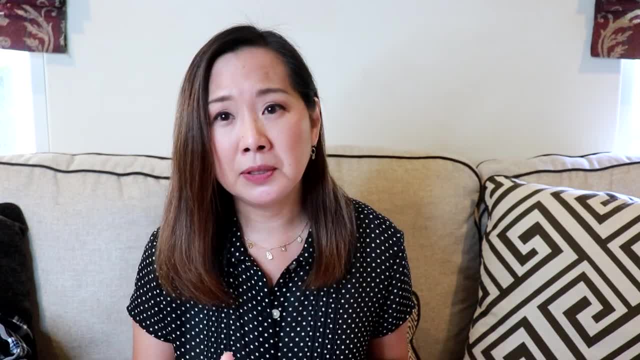 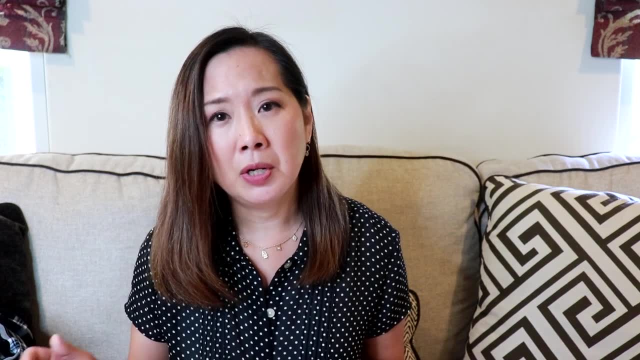 which is kind of an exact number. They typically use a two to three ratio, which breaks down to one to 1.5, or a three to five ratio, which breaks down to one to 1.7.. So yeah, I think you just have to use your judgment. 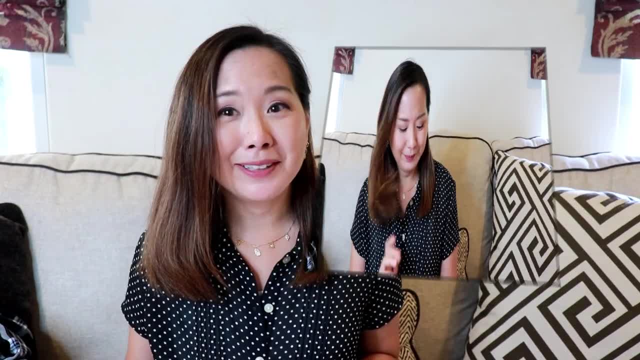 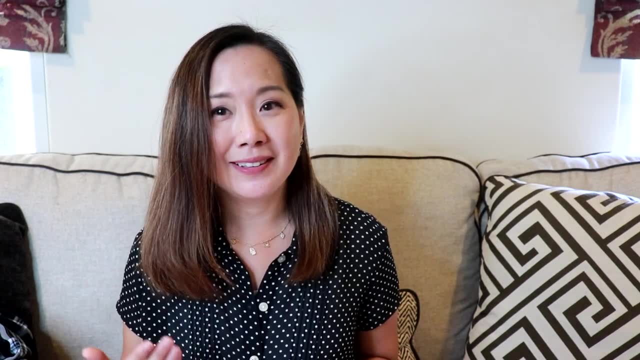 but it's just basically kind of a guide. Okay, So now that I've quickly explained what the golden ratio is and how it can help you to dress better, I'm going to go ahead and see if it actually works. So I'm going to put it into practice. 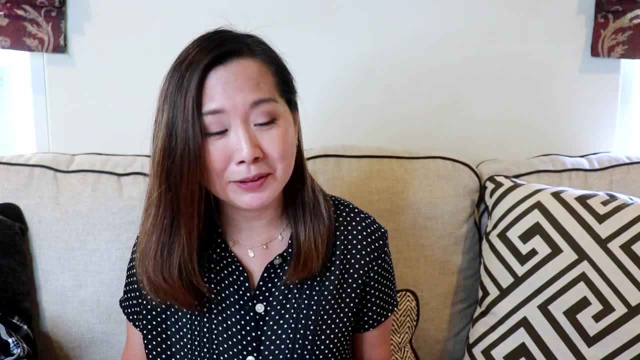 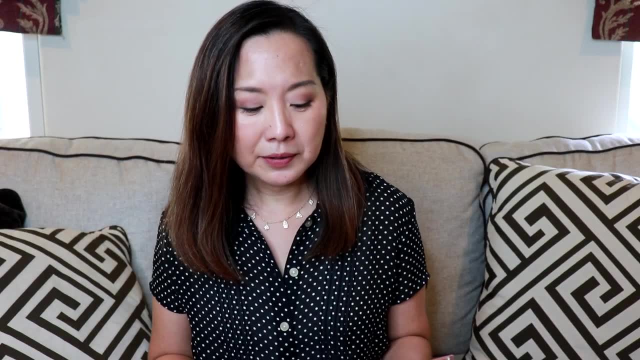 by trying to create three outfits using this golden ratio and to see if they actually look good. All right, let's see. Okay, So I went to my closet and tried to come up with some outfits that would put this golden mean ratio rule. 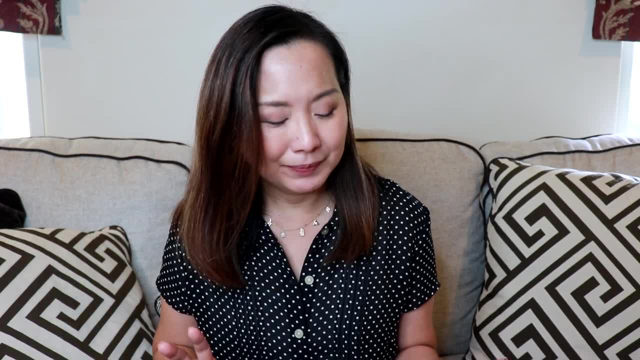 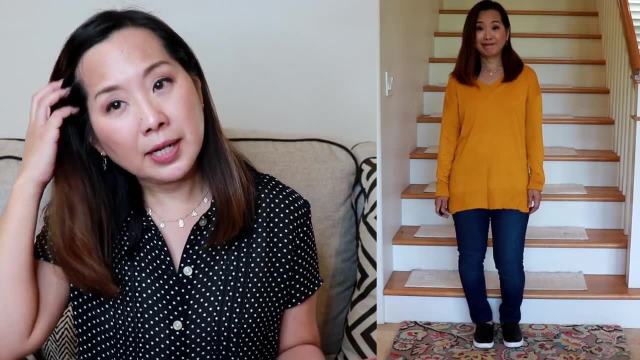 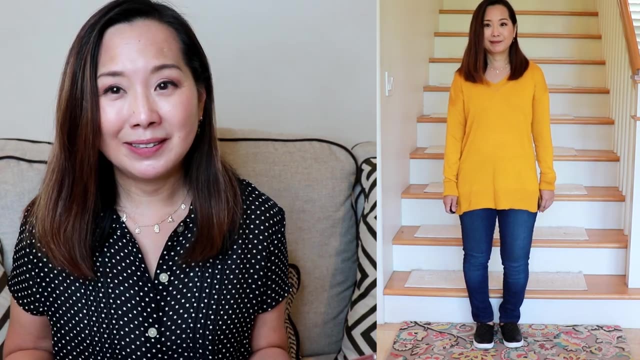 to the test. Okay, So first up, I paired a tunic length sweater, a pair of jeans and I just had black flats. So, as you can see in the picture, it pretty much cuts me off. So I don't think that. 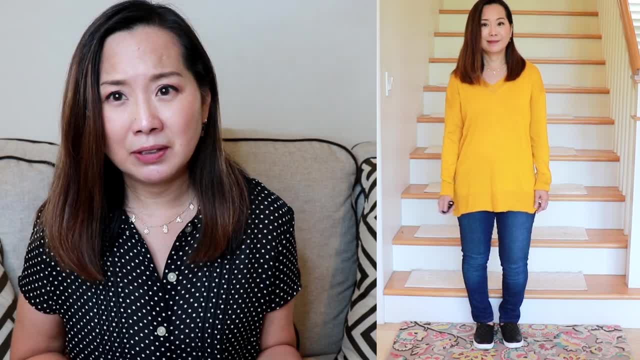 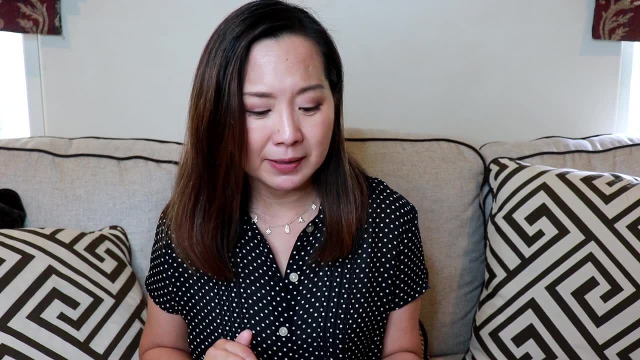 is the most flattering look, but it's probably something that I would have probably worn anyway. Hmm, But according to the golden mean ratio, yes, a one-to-one is not the most flattering, So to adjust it to more of a golden mean ratio. 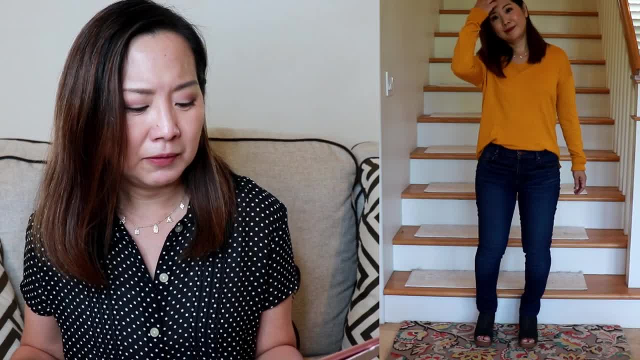 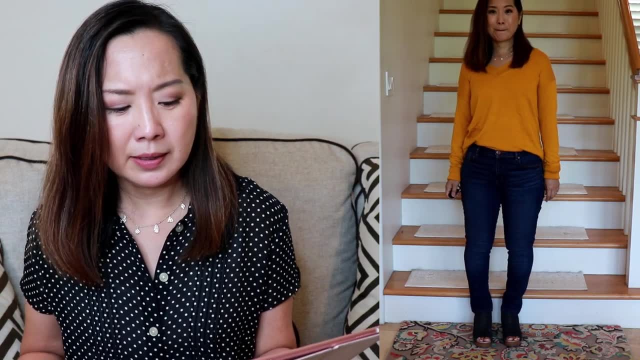 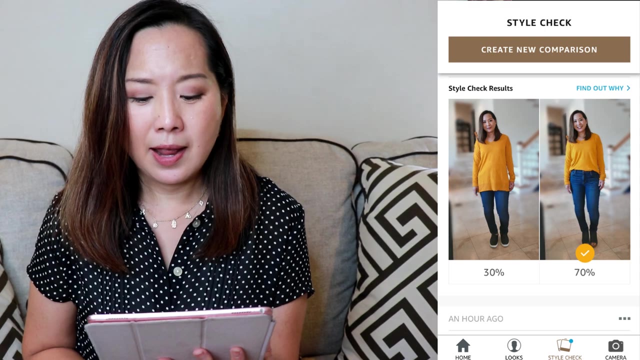 I did a front tuck and I also added a pair of higher shoes, So these are like wedge peep toe sandals And, yeah, I think that does look more attractive. And also what I did was I used my echo look to do a style check on this. 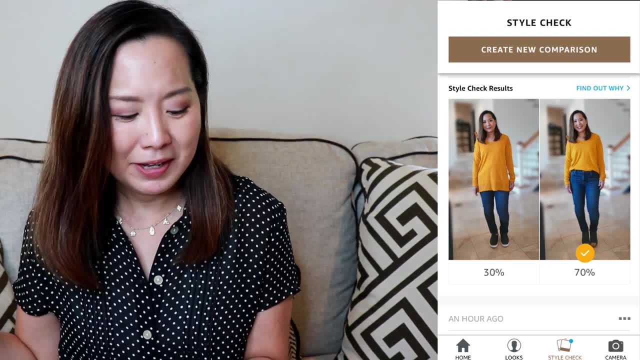 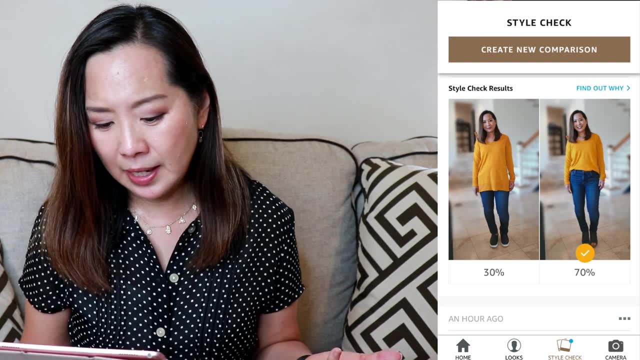 And it said that the golden mean ratio outfit was a lot better. So yeah, I would say that this is a more flattering look. I can just tell by looking at the picture right away. And yeah, So I would say, if you wanted to wear. 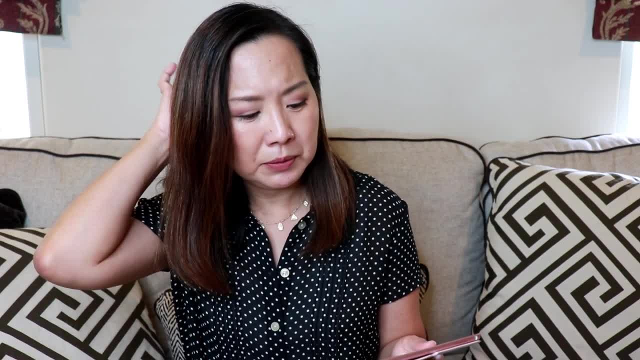 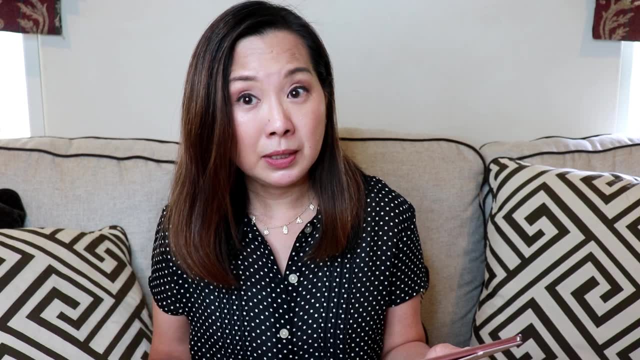 a tunic length sweater. it is kind of challenging for someone like me who's only 5'1", but you could just add heels. I think it would still look okay. It would look definitely better. It wouldn't hit the golden mean. 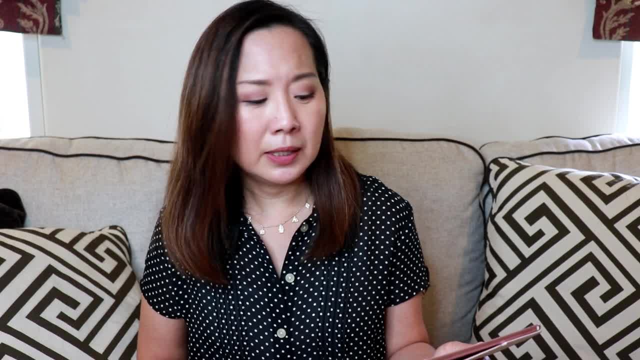 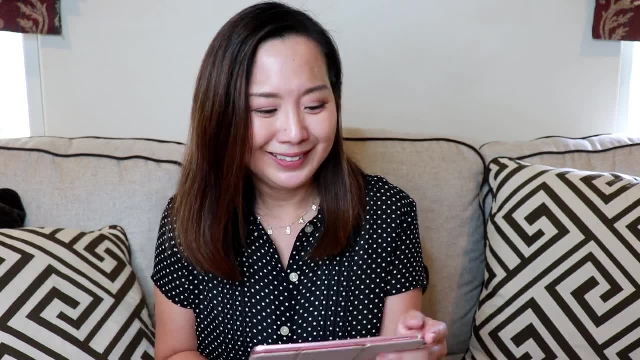 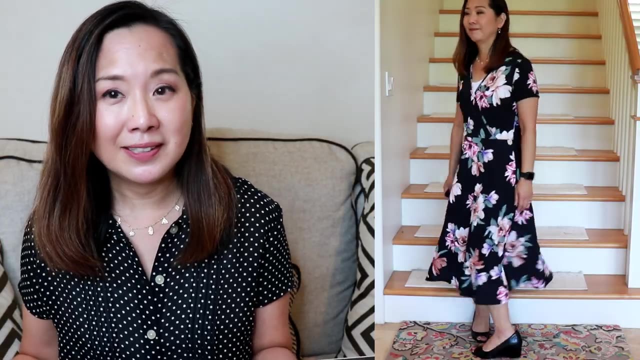 but it wouldn't be one-to-one, Or you could try to get like a tunic length sweater that maybe is just a couple inches shorter. I think that could work. Yeah, If you're tall, no problem. Okay, and next I tried comparing a longer dress. 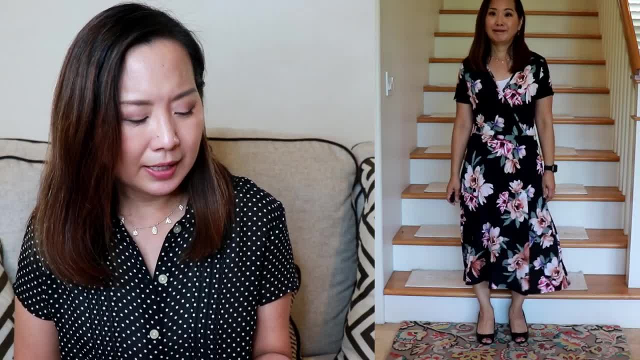 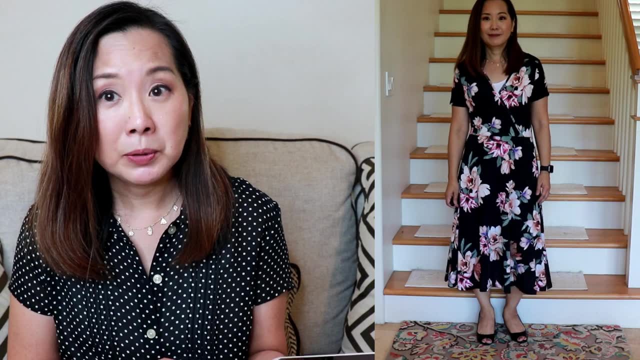 and I actually don't have too many of those. I was checking through my wardrobe and I must've gotten rid of the ones that I had, So this is one that I recently got from the from Golden Tote that I actually really like. 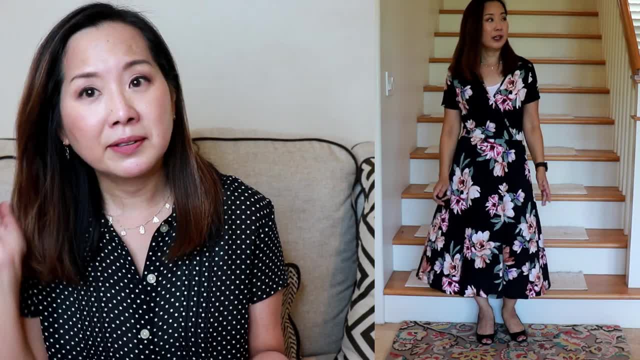 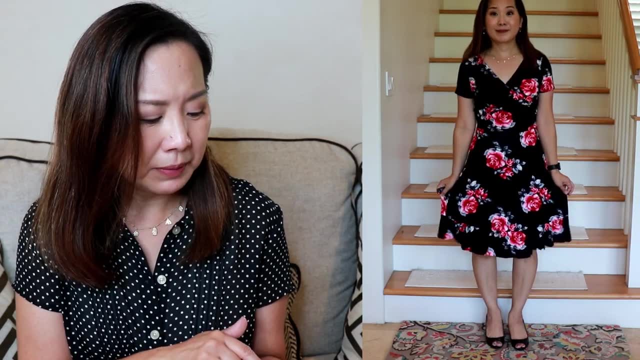 but it is kind of on the longer side. It's not quite a maxi but more of a midi length. So I compare that to another dress that I had gotten recently from Mix and Match. That's kind of a similar kind of faux wrap style. 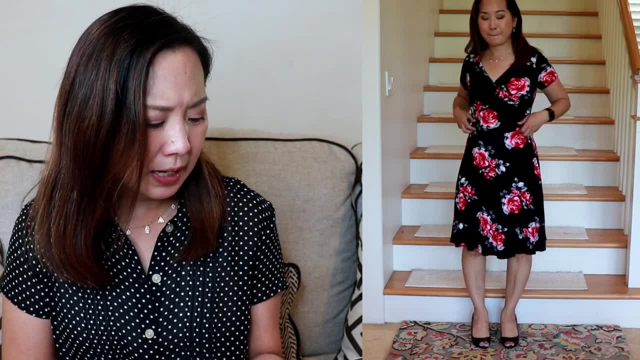 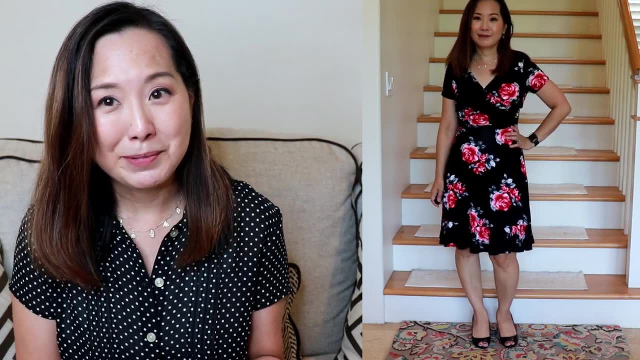 little bit different print, but the size of the flowers is about the same. This one's considerably shorter, though. It's about a little bit above the knee, And although that isn't the golden mean ratio ideal length, I mean it's supposed to be a lot shorter than that. But in this case I also put it to the test And, as you can see, the golden mean ratio-ish dress, which is, with the shorter hemline, the longer style. So yeah, so I think for me the shorter hemline looks better. 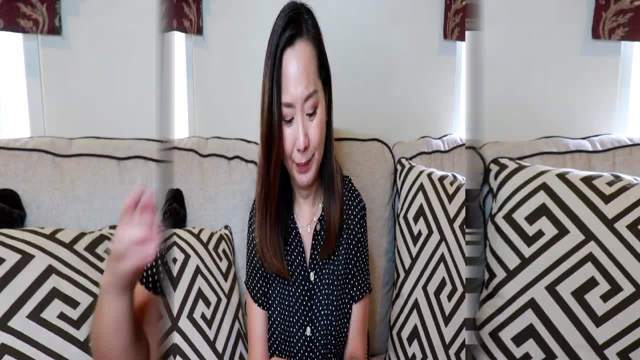 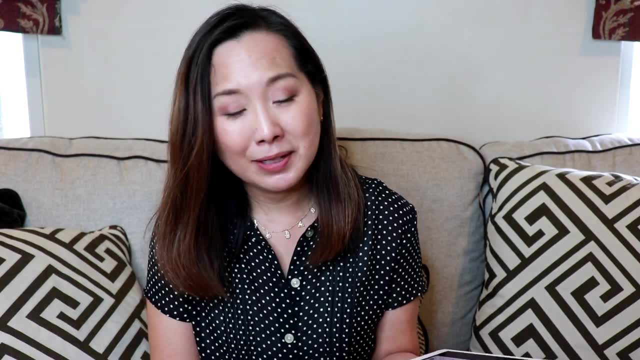 Okay, and for my last outfit, I have this one skirt, and this one is also a longer skirt, but I thought I'd try applying the golden mean, because it actually could be applied to your height, but it also could be applied to your pieces of clothing. 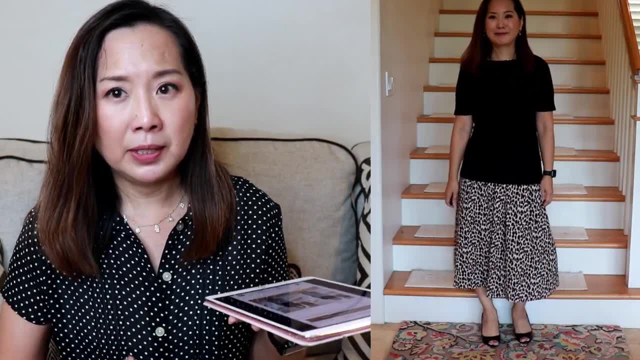 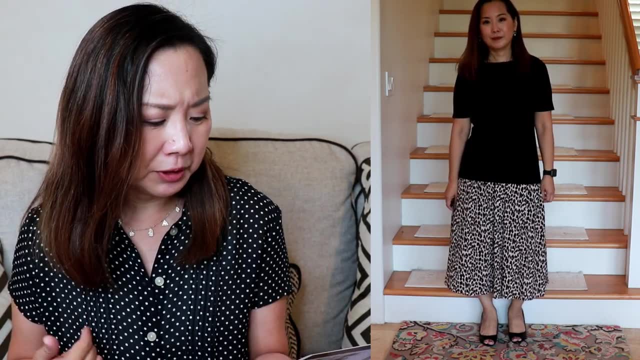 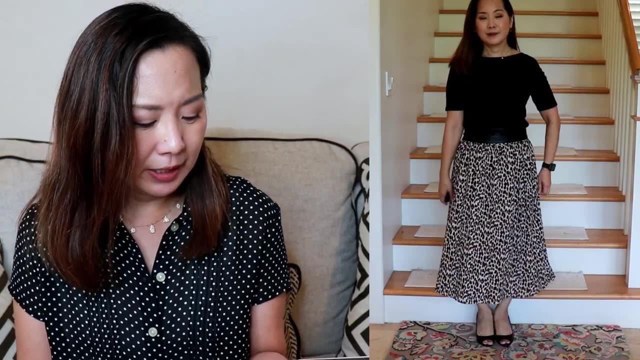 as compared to each other. So in this case I'm comparing the shirt. I have a black t-shirt and skirt, So when I wear it out it's like it cuts off at a one-to-one ratio. So to adjust it to more of a golden mean ratio: 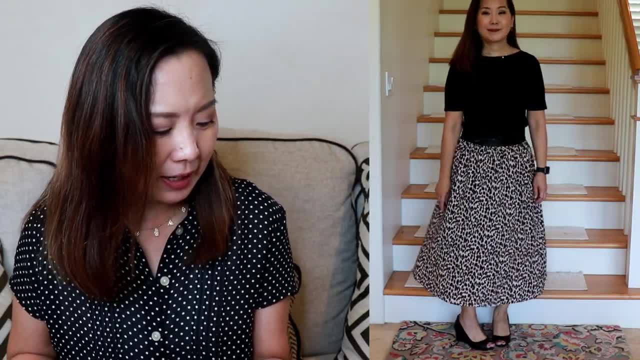 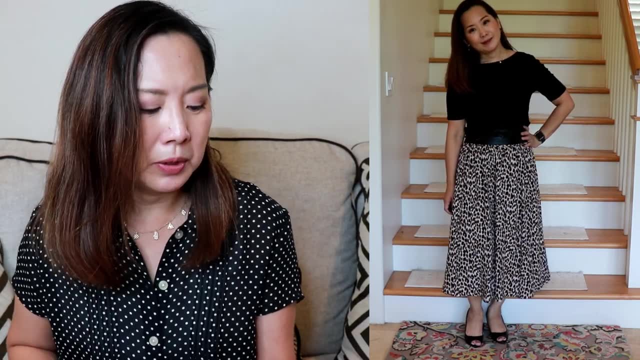 I tucked it in and then it was a little too short so I added a black belt, so you have more of the golden mean ratio, This one. I would say it's more like a one-to-1.5.. So that's still within margin of error, I think. And then I use my the golden mean outfit by now. So that's it for this video. I hope you enjoyed it And I'll see you in the next one. Bye.